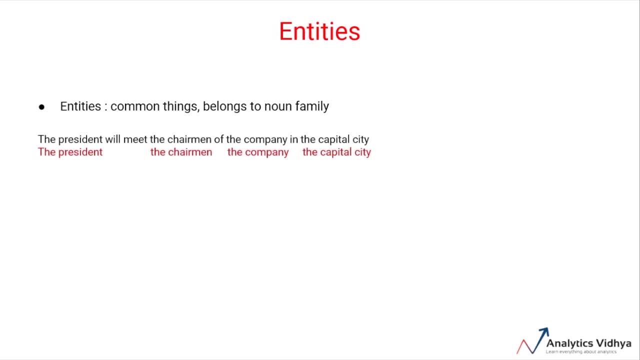 in the sentence. For example, consider a sentence: the president will meet the chairman of the company in the capital city. In this sentence, the entities are the president, the chairman, the company and the capital city, because these phrases represent common things such as persons, locations etc. 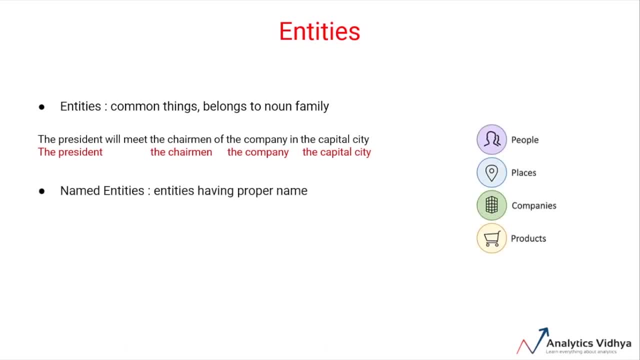 So what are named entities? Those entities in the text having proper noun as the part of speech tags and having proper naming are called named entities. For example, consider an alternate sentence: Donald Trump will meet the chairman of Google in the New York City. 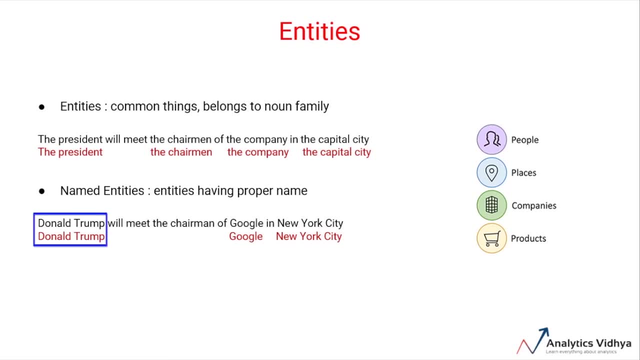 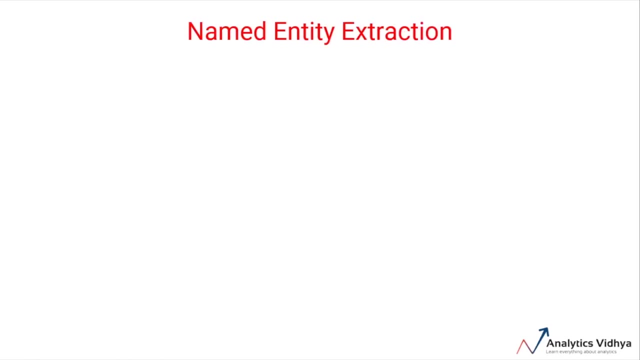 In this case, the entities are Donald Trump, the chairman, Google, New York City, but the named entities are Donald Trump, Google and New York City because these entities have proper names and have proper noun as the part of speech tag. Named entity extraction is a step-by-step process. 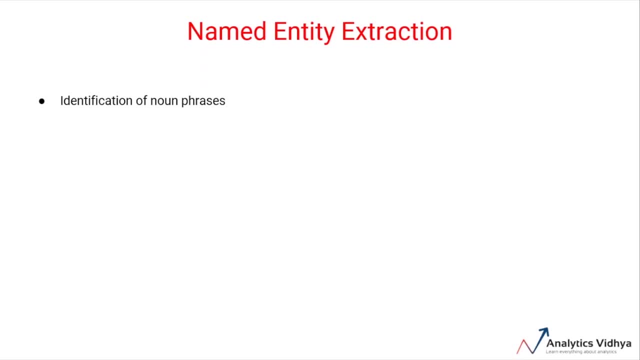 to find those noun phrases from text data which are also named entities. One of the key property of noun phrases is that they are connected to the root of the noun. So if you have a noun phrase of a tree or a smaller sub-tree in the dependency graph by direct object or direct subject, 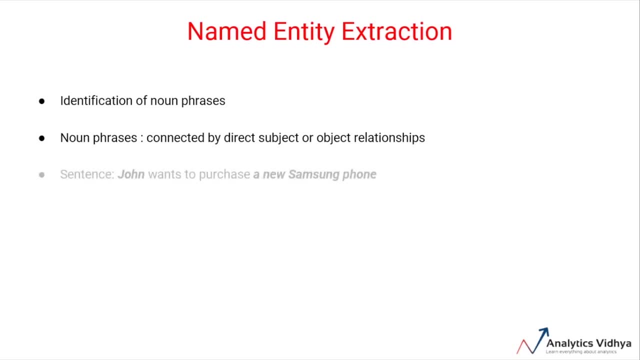 relationships. For example, consider the sentence John wants to purchase a new Samsung phone. The dependency graph of this sentence will look something like this, in which the word purchase is the main verb and it acts as the root of the sentence. This root has three leaves. 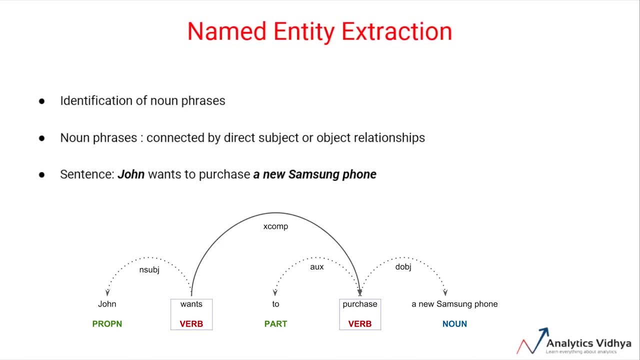 One corresponds to the word wants, connected by the complementary relation. Second leaf is connected by the auxiliary relation to word to. and the third connection is not a leaf, It's a phrase corresponding to a new Samsung phone, connected by the direct object relation. This means that object phrase or one of the noun phrase of this sentence. 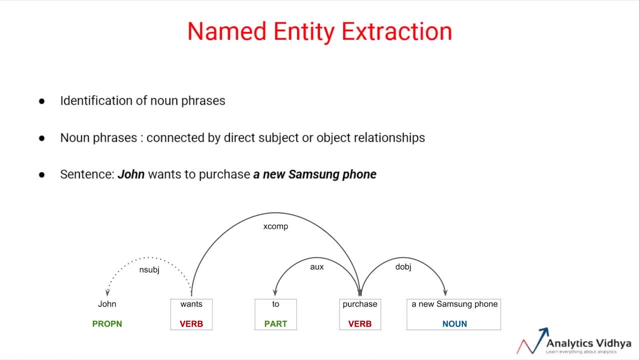 is a new Samsung phone. Further, the word wants is connected to John by noun subject relation, which indicates that John is subject. The word wants is also one of the noun phrase. So if we parse this tree, we can obtain two noun phrases: John and a new Samsung phone. If we now annotate this sentence with the